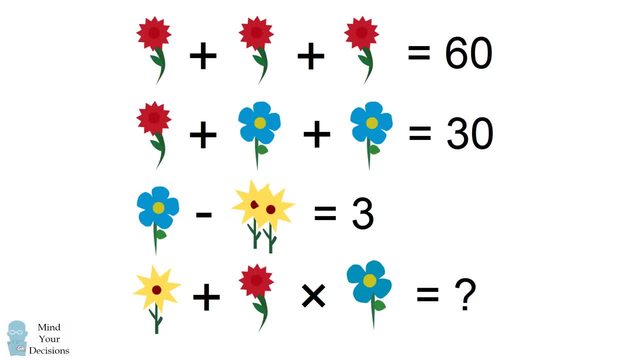 keep watching. In this video, I will present what many people consider to be the correct answer. To get started, you want to look very closely at the pictures. In the very last equation, the first picture shows one yellow flower. This is not the same as the equation before, which has two yellow flowers. 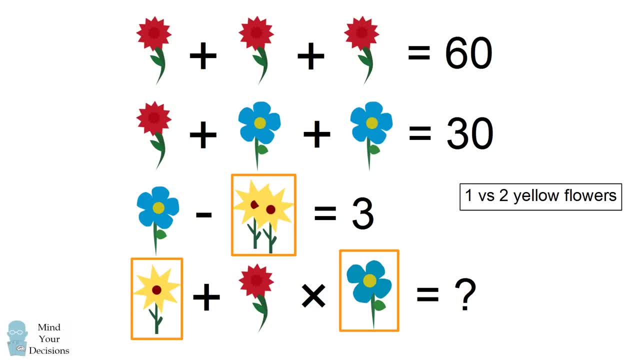 Now look at the blue flower. in the last equation There are four petals on this flower. In all of the other blue flowers there are five petals. Arguably, these differences mean that the very last equation cannot be evaluated. However, we can try and assign a consistent value with all of the other information in this problem. 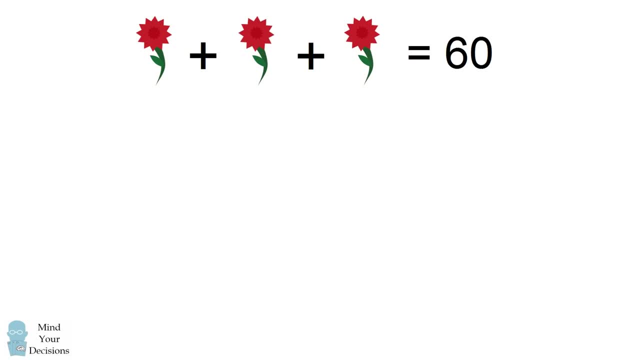 Let's try and do that. The first equation has three red flowers equal 60. This means one red flower is equal to 20. to 20.. The next equation has a red flower plus two blue flowers equal 30. We can use the value of 20 for the red flower and then we have 20 plus two blue. 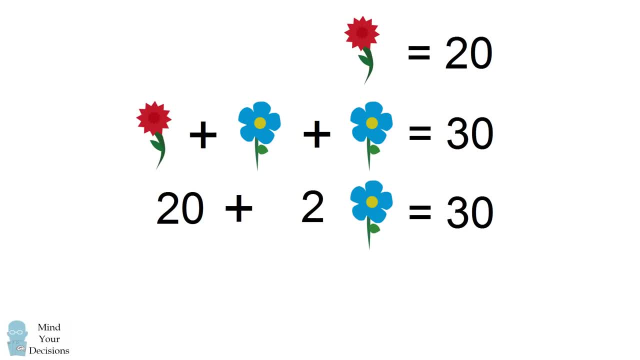 flowers with five petals equal to 30. We subtract 20 from both sides, so we have two blue flowers with five petals equaling 10.. If we count each petal as a value, we have a total of 10 blue petals. So we can assign a value for a blue. 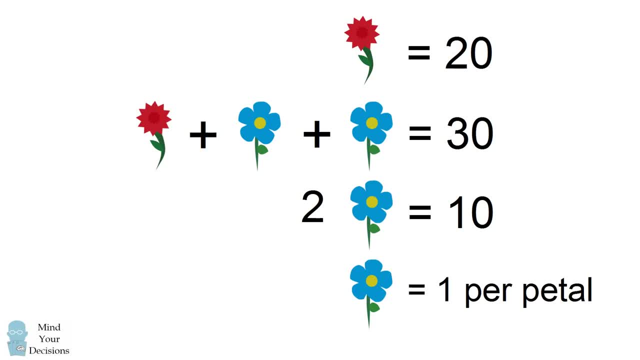 flower as saying it's equal to one per petal. The next equation has a blue flower with five petals minus two yellow flowers, equal to three. We can assign the blue flower with five petals a value of five. We then are subtracting two yellow flowers to be equal to three. This means that each 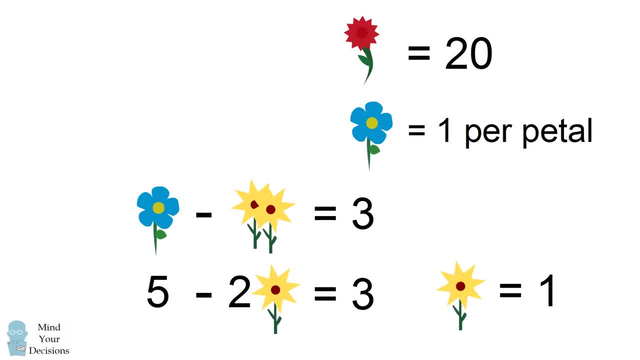 yellow flower has a value of one. Now we'll use this information to try and evaluate the last expression. the yellow flower will replace with the value of one, the red flower will replace with the value of 20 and the blue flower with four petals will replace with the value of 4.. We have 1 plus 20.